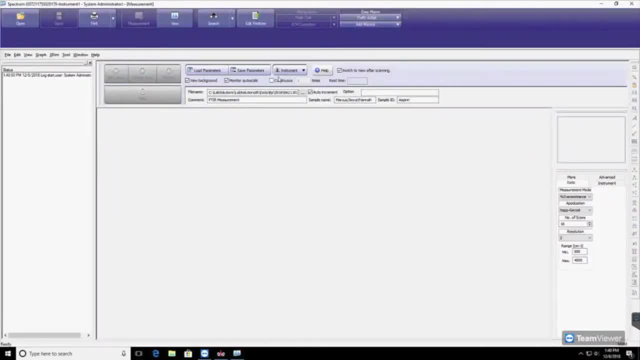 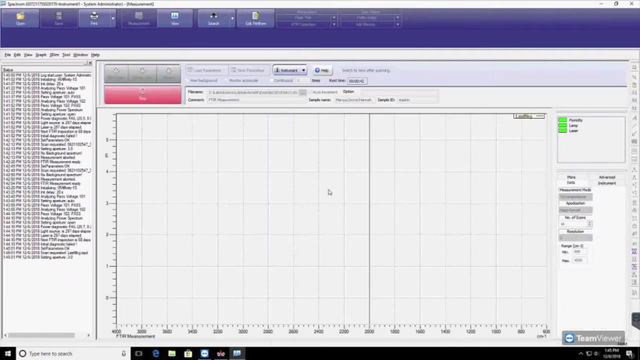 program located on the desktop Under the instrument tab, select initialize. You may receive an error message. Click yes to continue. Once the initiation is complete, perform a background scan by clicking on BKG scan. An IR will appear. Click OK. 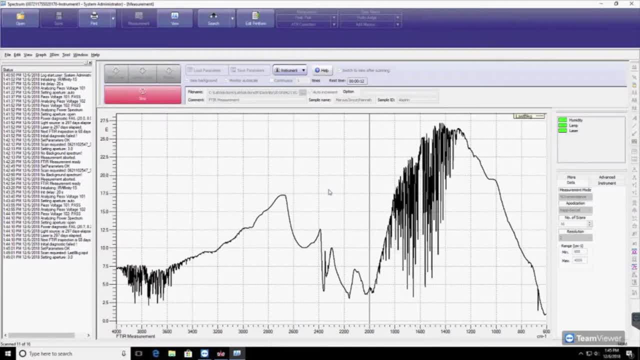 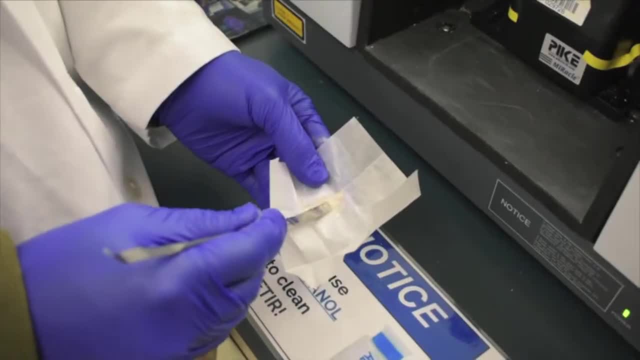 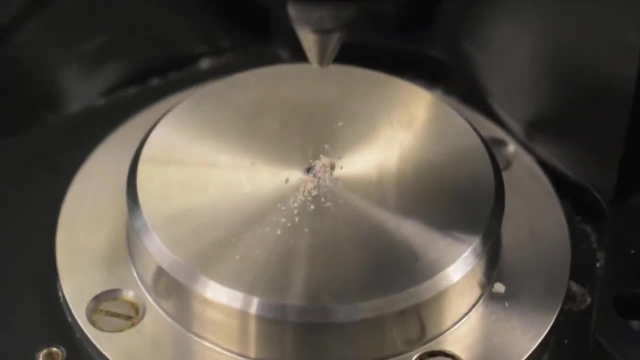 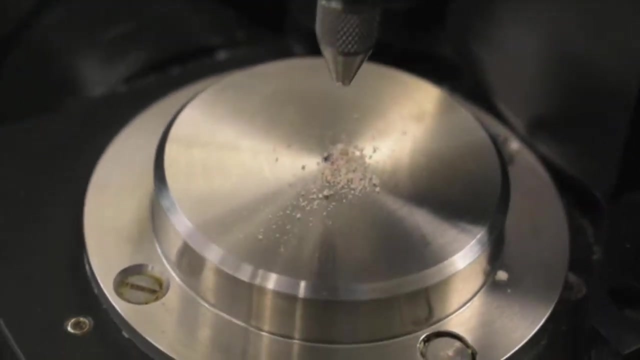 When the background scan is done, you can now scan your sample. Use the spatula to transfer your dry sample onto a loading tray. Once the initiation is completed, perform a background scan by clicking on BKG scan. The knob should be rotated until you can hear a single loud click. 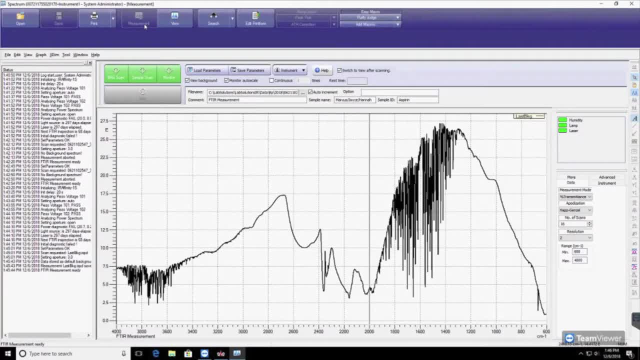 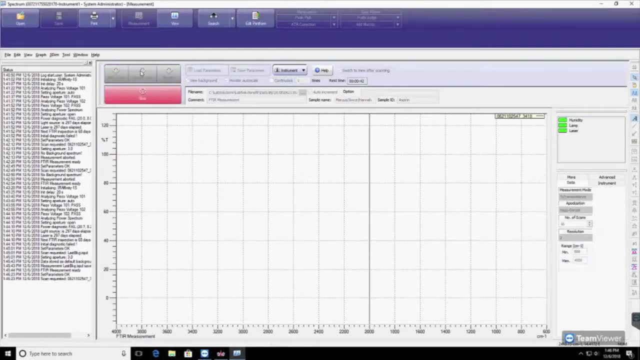 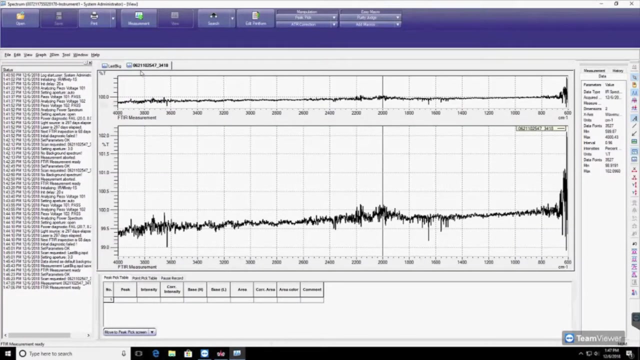 Show augment engaging the computer. Click on measurement and select sample scan. Once the scan is complete, you can label the peaks by going to the menu located here and select on auto cursor. And that's it. Thanks for watching, Bye. Move the cursor to the peak in my label and click. 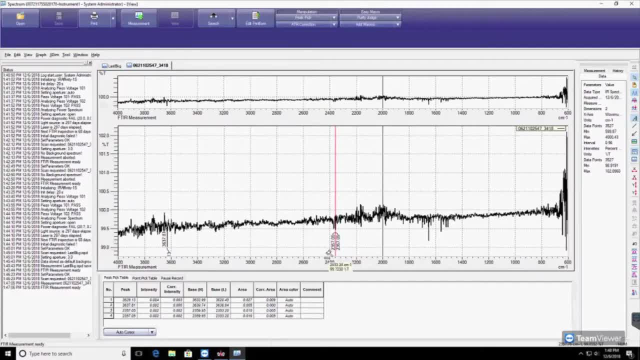 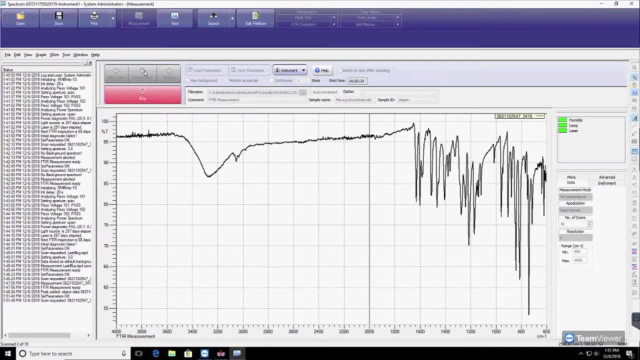 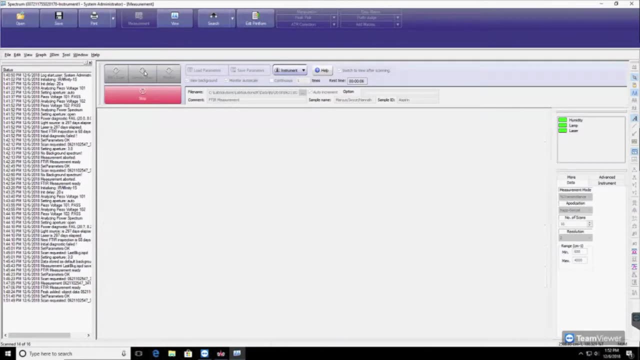 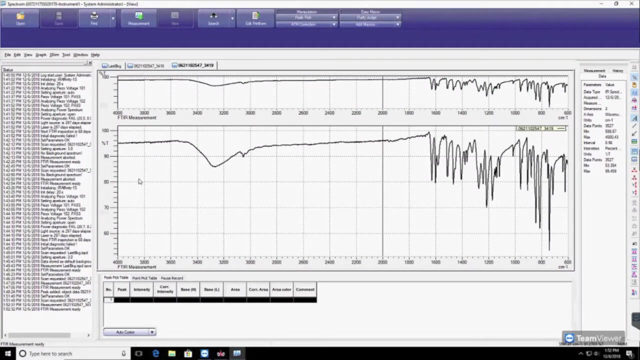 You can also select a range of peaks by dragging the cursor. Let's test your knowledge and see what you've learned so far. What color are the unicorns? Pink. Where are they dancing? Are they dancing on rainbows? Please use one word to describe the texture of their magical fur. 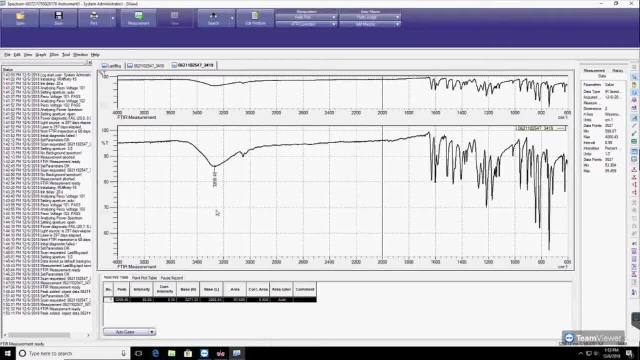